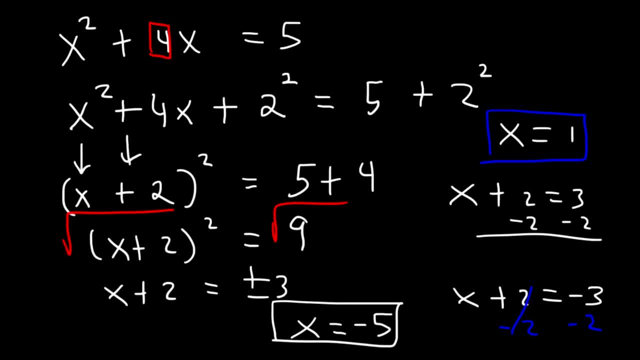 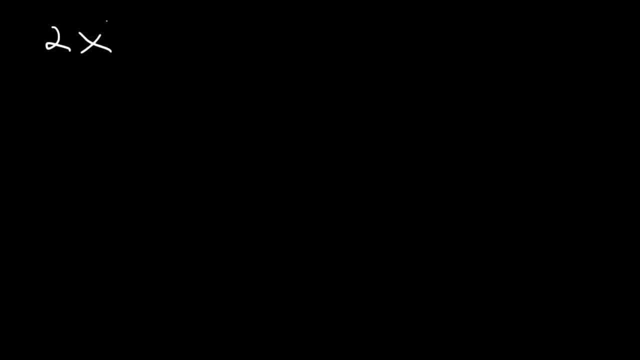 So x is equal to negative 5.. Now let's work on another example. Try this one: 2x squared minus 12x minus 7 equals 0.. Solve by completing the square. So first I'm going to move the negative 7 to the right. 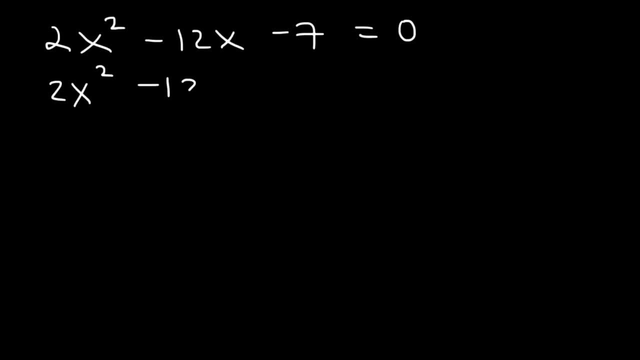 So 2x squared minus 12x is equal to positive 7.. Now notice that there's a 2 in front of x squared. What we need to do is factor out the 2.. If we take out 2, it's going to be x squared minus 6x. 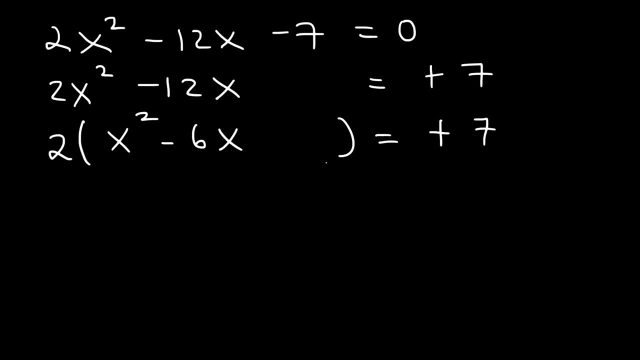 And then I'm going to leave a space. Now let's complete the square. Half of 6 is 3. And we need to square it. So I value, I added not just 9 to the left side, but 9 times 2,, which is 18.. 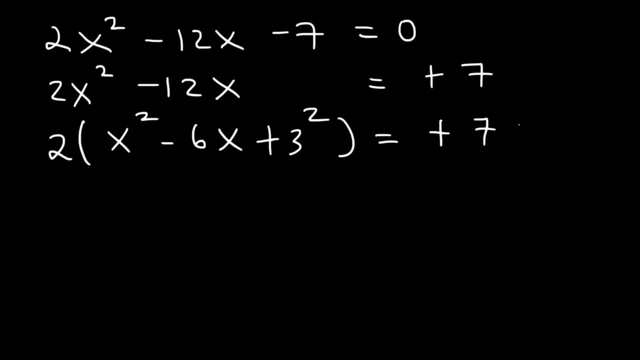 Now, whatever you do to the left side, you must also do to the right side. So I have to add positive 18 to the right side. Now to factor x squared minus 6x plus 3 squared, it's going to be x. whatever this symbol is minus this number squared. 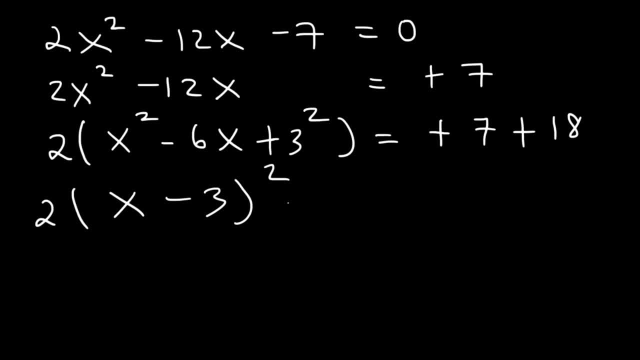 x squared minus 6x plus 9 is x minus 3.. And then 7 plus 18, that's 25.. Now let's divide by 2.. So x minus 3 squared is equal to 25 divided by 2.. 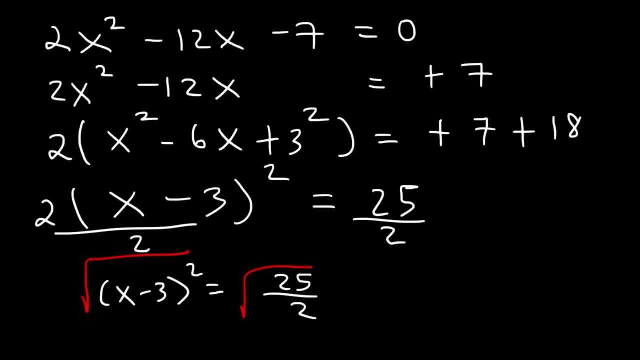 Now we can take the square root of both sides. So on the left it's just going to be x minus 3.. On the right, plus or minus, the square root of 25 is 5.. The square root of 2, we'll just leave it as root: 2.. 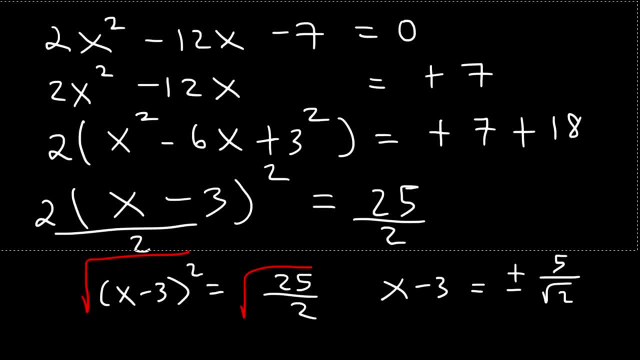 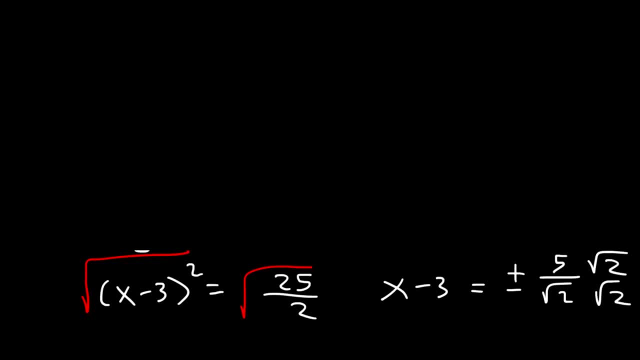 Now let's rationalize this expression. Let's multiply the top and the bottom by root 2.. So x minus 3 is equal to plus or minus 5 root 2 over 2.. Now all we can do now is just add 3 to both sides. 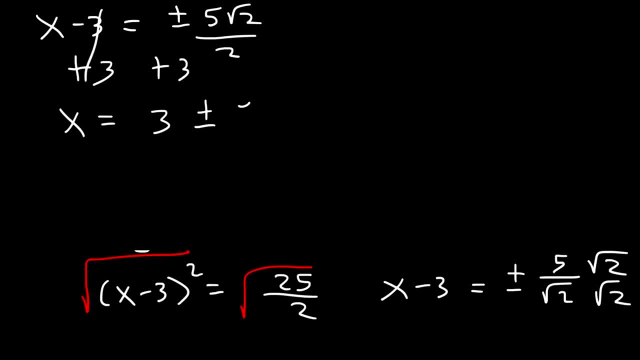 So x is equal to 3 plus or minus 5 root 2 over 2.. Now we can't add 3. And 5 root 2 over 2. We can't add them together, So we're just going to leave it like this. 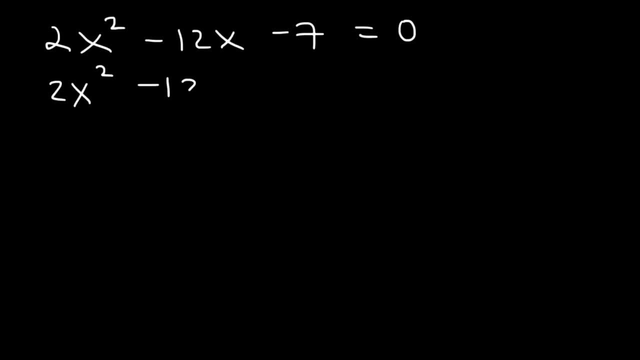 So 2x squared minus 12x is equal to positive 7.. Now notice that there's a 2 in front of x squared. What we need to do is factor out the 2.. If we take out 2, it's going to be x squared minus 6x. 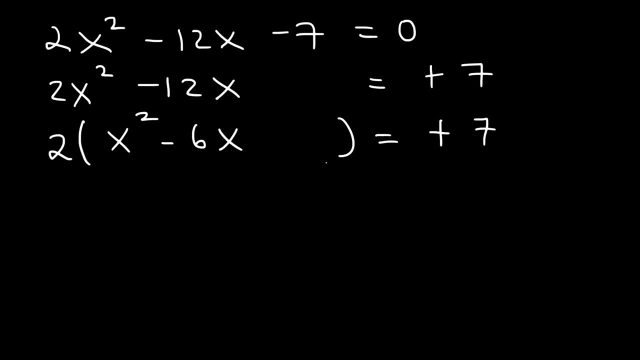 And then I'm going to leave a space. Now let's complete the square. Half of 6 is 3. And we need to square it. So I value, I added not just 9 to the left side, but 9 times 2,, which is 18.. 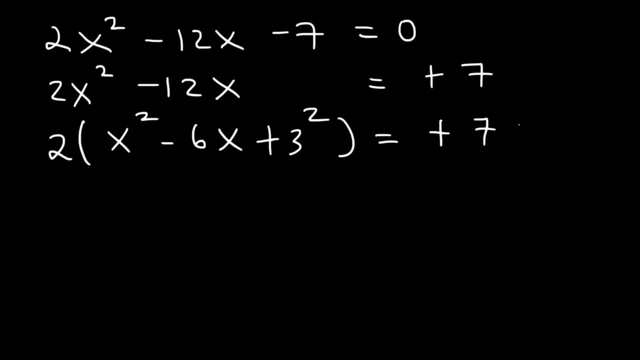 Now, whatever you do to the left side, you must also do to the right side. So I have to add positive 18 to the right side. Now to factor x squared minus 6x plus 3 squared, it's going to be x. whatever this symbol is minus this number squared. 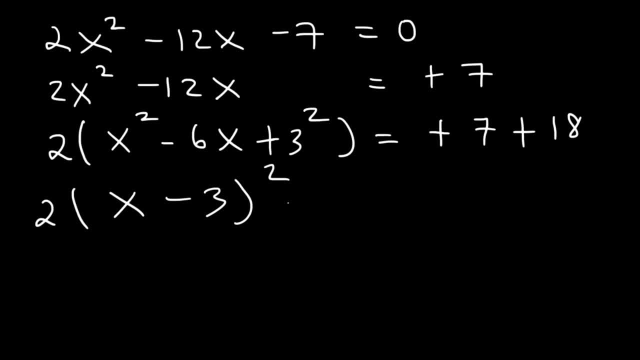 x squared minus 6x plus 9 is x minus 3.. And then 7 plus 18, that's 25.. Now let's divide by 2.. So x minus 3 squared is equal to 25 divided by 2.. 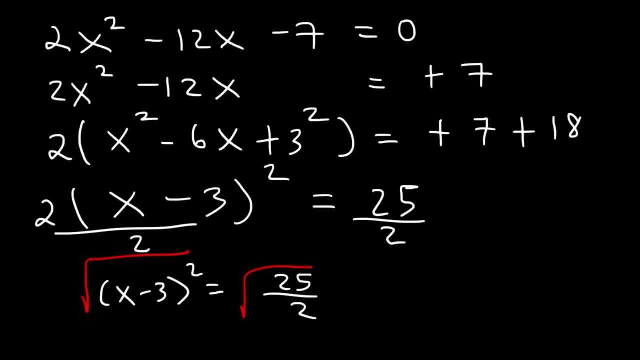 Now we can take the square root of both sides. So on the left it's just going to be x minus 3.. On the right, plus or minus, the square root of 25 is 5.. The square root of 2, we'll just leave it as root: 2.. 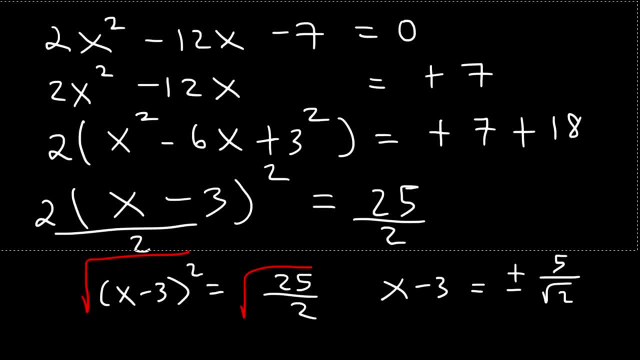 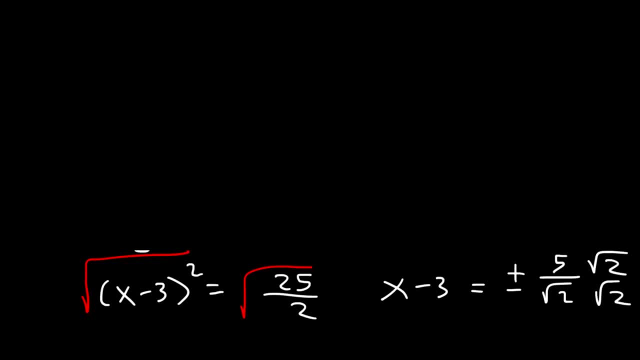 Now let's rationalize this expression. Let's multiply the top and the bottom by root 2.. So x minus 3 is equal to plus or minus 5 root 2 over 2.. Now all we can do now is just add 3 to both sides. 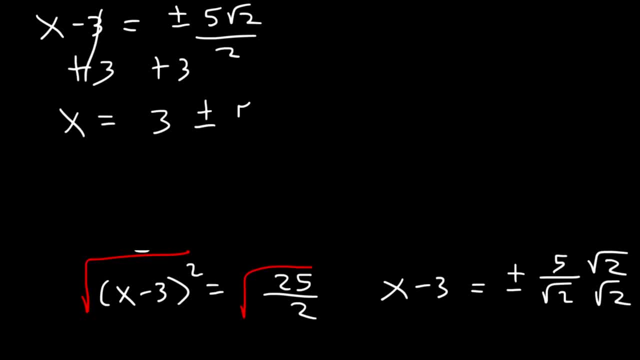 So x is equal to 3 plus or minus 5 root 2 over 2.. Now we can't add 3. And we can't add 2.. We can't add 2.. 5 root 2 over 2.. 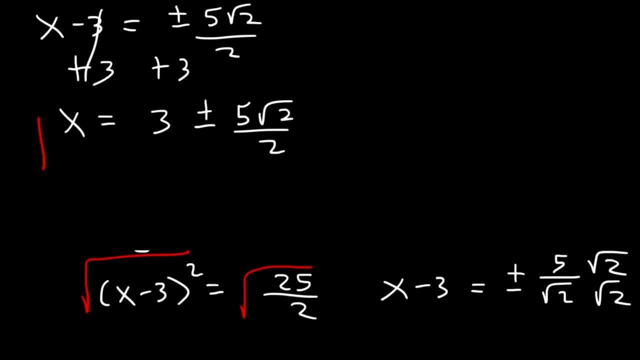 We can't add them together, So we're just going to leave it like this. This is the answer. Now, keep in mind there's two answers. The first answer is 3 plus 5 root 2 over 2.. And the second answer is 3 minus 5 root 2 over 2.. 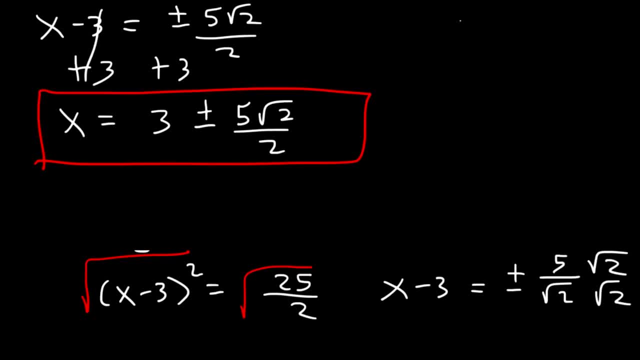 This is the answer. Now, keep in mind, there's two answers. The first answer is 3 plus 5 root 2 over 2.. And the second answer is 3 minus 5 root 2 over 2.. Now let's try another example. 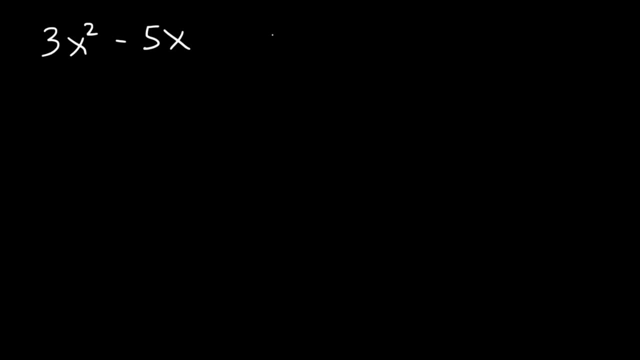 3x squared minus 5x is equal to 10.. Solve by completing the square. Now the first thing we're going to do is take out a 3x From the first two terms. 3x squared divided by 3 is x squared. 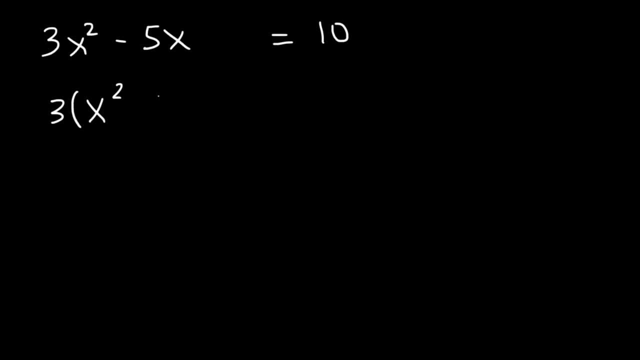 Negative 5x divided by 3.. Well, it's just going to be negative 5 over 3x. Now we need to take half of this number. Half of 5 over 3 is basically 5 over 6.. Multiply the denominator by 2.. 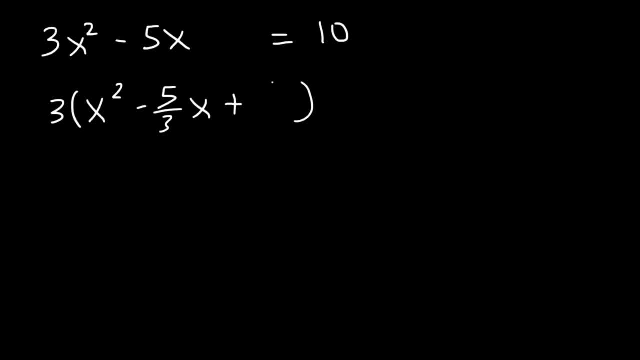 That's how you can find a half of a fraction And then, once we take half of it, we need to square it, So it's going to be 5 over 6 squared. Now on the left side we've added 5 over 6 squared, but time stream. 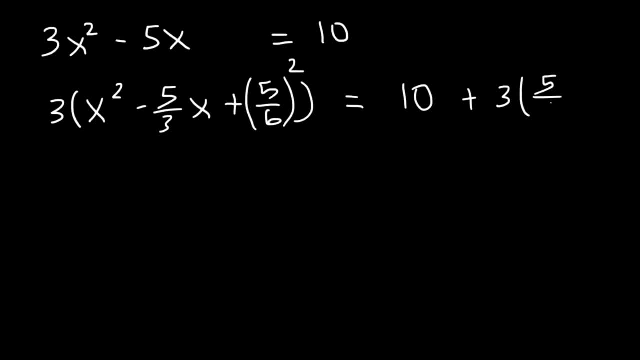 So we've got to add that to the right side as well. Now, how can we factor this expression? Everything you need. you can see it: It's going to be x and then, whatever this sign is, minus this number. before you square it. 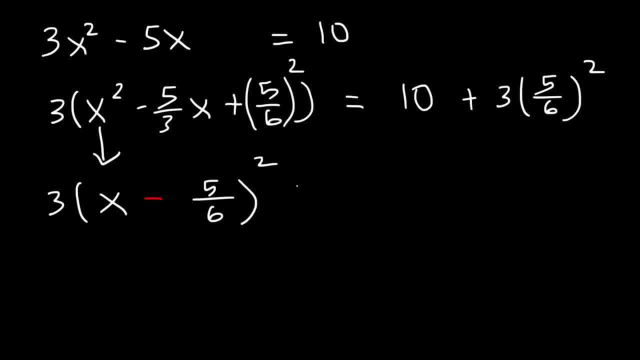 5 over 6 squared. It's always going to work out that way. On the right we have a 10 plus 3. 5 squared is 25.. 6 squared is 36.. Now let's combine this first. 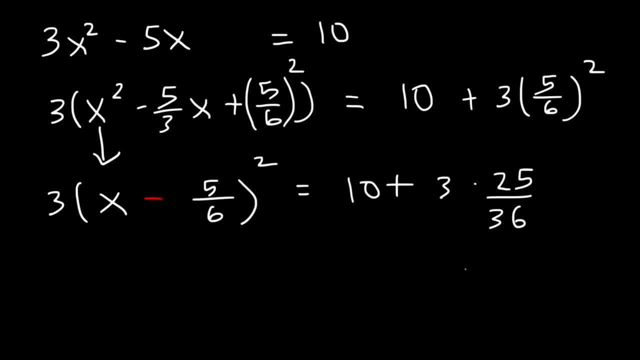 3 over 36.. If we divide 36 by 3, we're going to get 12.. So this is the same as 25 over 12. Plus 10 over 1.. Now let's take a look at this. 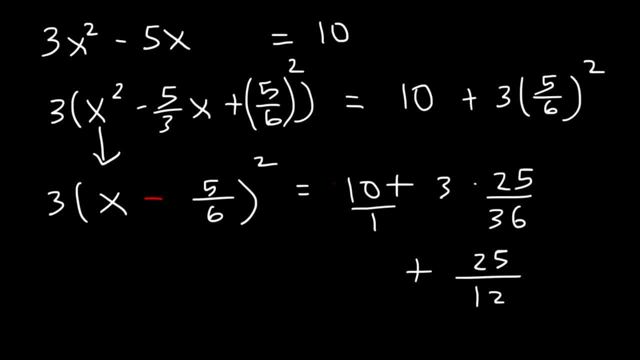 Let's take a look at this. Let's take a look at this. Let's combine 10 over 1 and 25 over 12.. To do that, we need to get common denominators. Let's multiply this by 12 over 12.. 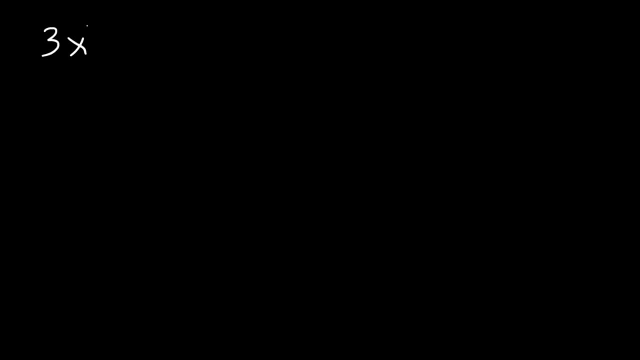 Now let's try another example. 3x squared minus 5x is equal to 10.. Solve by completing the square. Now the first thing we're going to do is take out a 3 from the first two times. We're going to use a 3.. 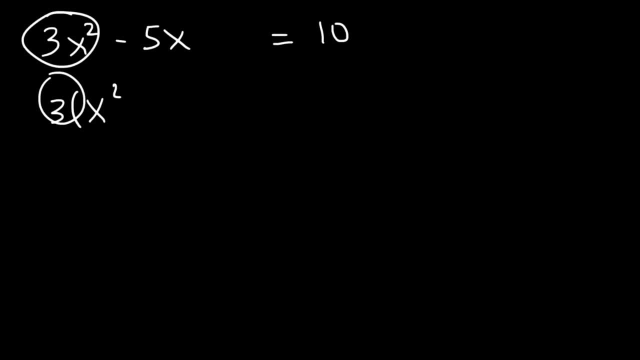 We're going to use a 3.. 3x squared divided by 3 is x squared Negative. 5x divided by 3, well, it's just going to be negative 5 over 3x. Now we need to take half of this number. 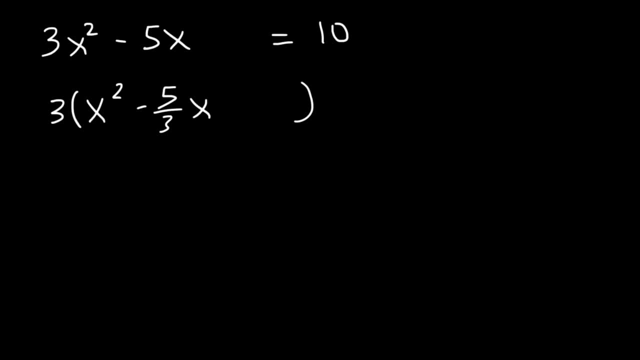 Half of 5 over 3 is basically 5 over 6.. Multiply the denominator by 2.. That's how you can find a half of a fraction, And then, once we take half of it, we need to square it, So it's going to be 5 over 6 squared. 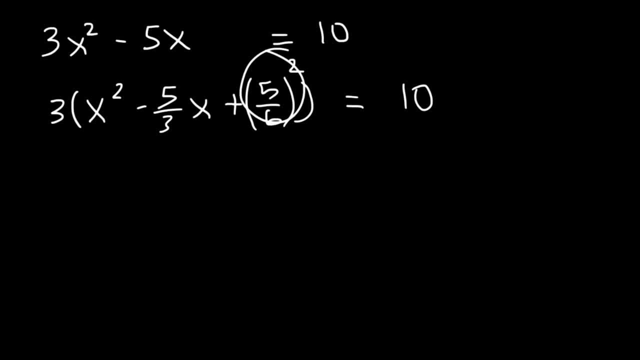 Now on the left side, we've added 5 over 6 squared, but time stream, So we've got to add that to the right side as well. Now how can we factor this expression: Everything you need. you can see it. 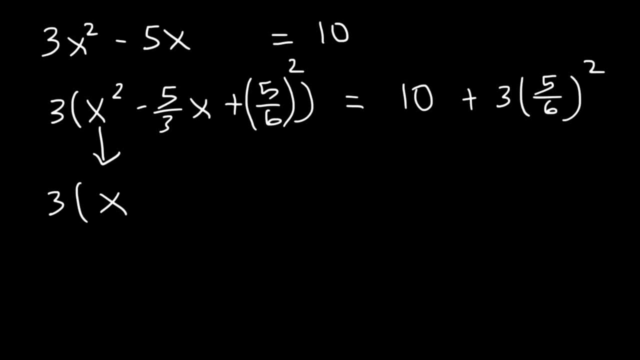 It's going to be x. and then, whatever this sign is, minus this number. before you square it: 5 over 6 squared. It's always going to work out that way. On the right, we have a 10 plus 3.. 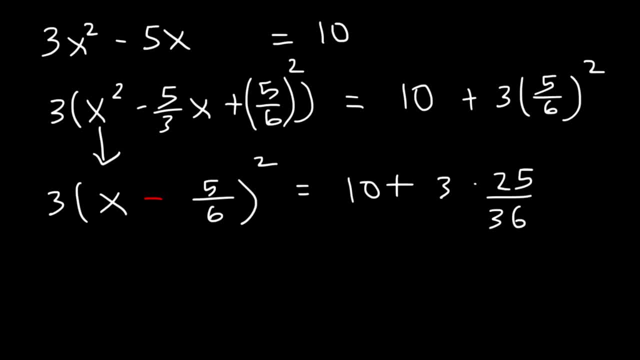 5 squared is 25.. 6 squared is 36.. Now let's combine this. first: 3 over 36.. If we divide 36. By 3, we're going to get 12.. So this is the same as 25 over 12.. 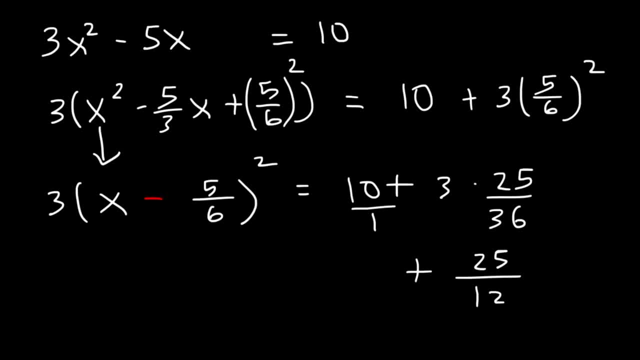 Plus 10 over 1.. Now let's combine 10 over 1 and 25 over 12.. To do that we need to get common denominators. Let's multiply this by 12 over 12. So that becomes 120 over 12.. 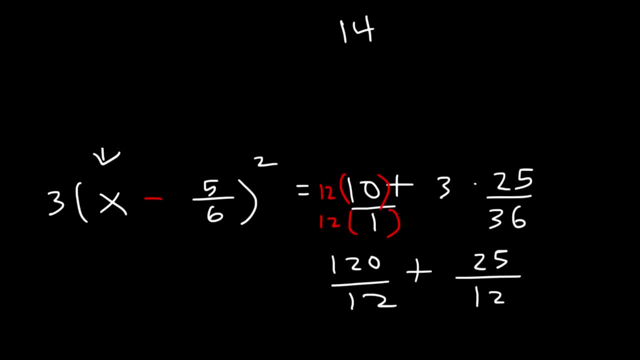 120 plus 25.. Is 145 over 12.. Now what we need to do is get rid of this 3.. So we're going to multiply both sides by 1 third. On the left side, 3 and 1 third will cancel.